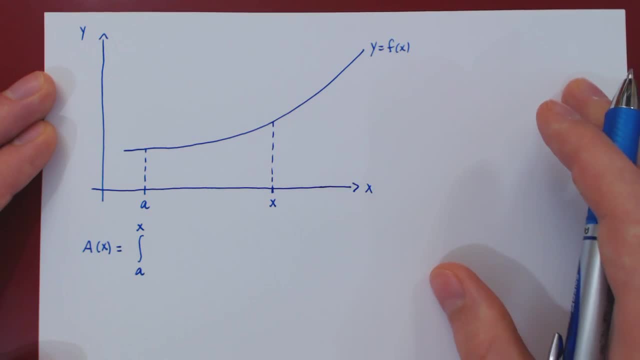 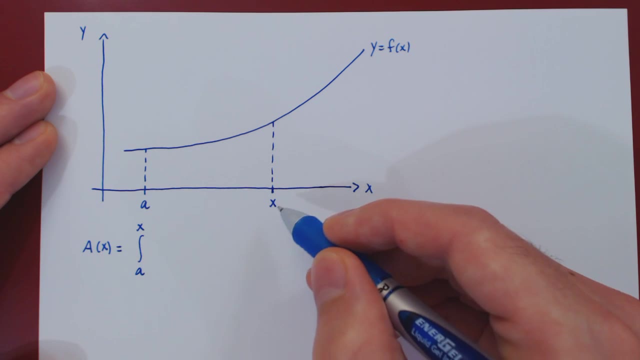 The one catch- and here's where we have to be careful- is we usually write the integral of f, of x, dx, But we are already using x As the variable right-hand point of the interval. so for the dummy variable of integration we have to use a different variable. 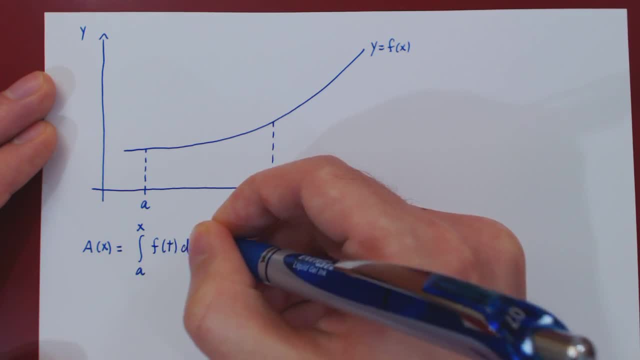 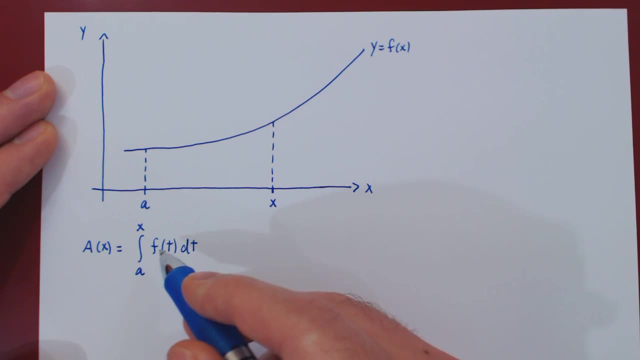 So let's go with t, so f of t dt. And again here, t is a dummy variable, so we could replace t by u, so f of u, du, or t by v, f of v dv. Any variable will do, but the variable x. 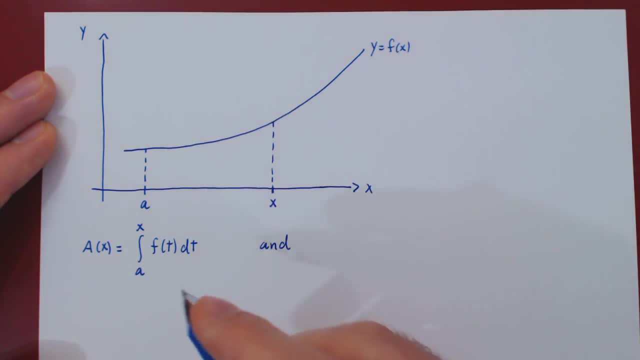 And since the function, Since the fundamental theorem of calculus connects the definite with the indefinite integral, let's write down also the indefinite integral of f, of x And again recall that the indefinite integral of lowercase f is asking for all of its antiderivatives. 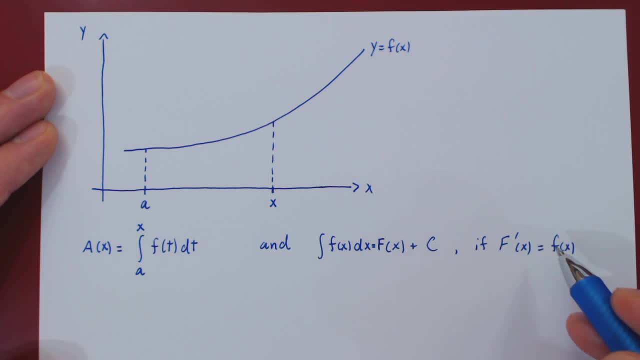 So all functions whose derivative is equal to lowercase f, And the key here is that antiderivatives are unique up to the addition of a constant right. When we write the integral of f of x, dx equals uppercase f of x plus c. 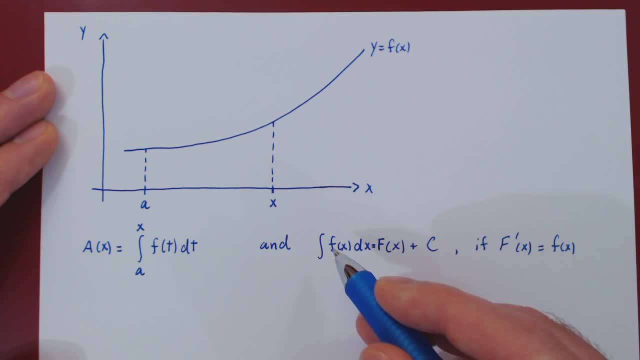 this represents again all antiderivatives to lowercase. So any antiderivative to lowercase f must be f of x plus some constant. So essentially, up to the addition of a constant, antiderivatives are unique And this will be the key to the argument. 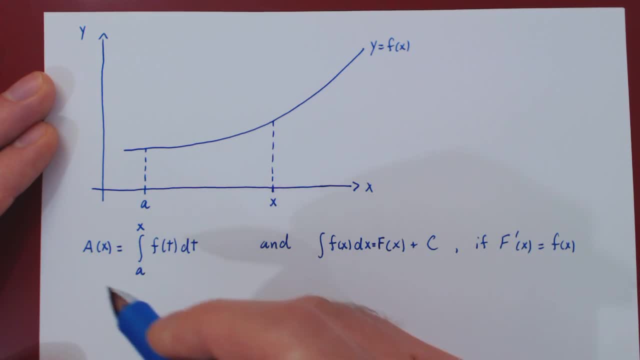 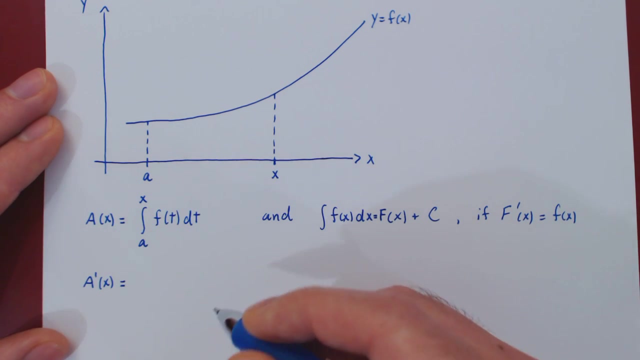 And now we want to show that the area function is actually an antiderivative to lowercase f. So we want to show that a prime of x equals f of x. And to show this, to find the derivative of the area function, we have to go back to square one. 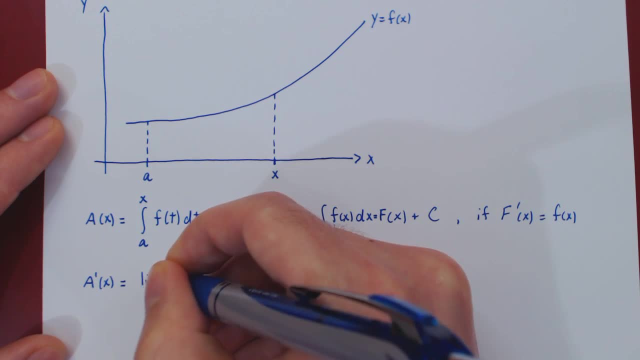 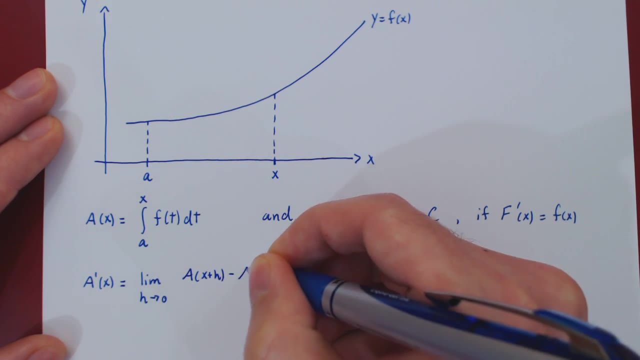 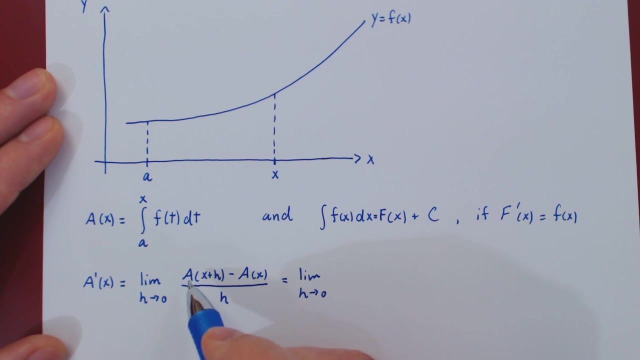 The definition of the derivative is the limit as h approaches zero, The function at x plus h minus the function at x over h. And now let's try to figure out what a of x plus h is right. This is the area below the function f, from a to x plus h. 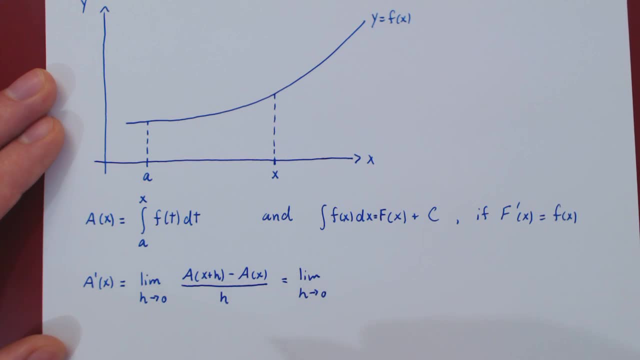 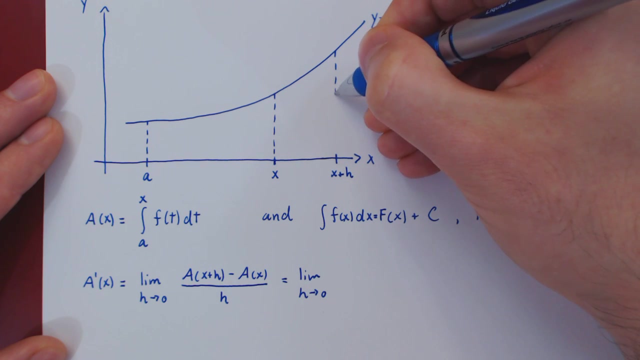 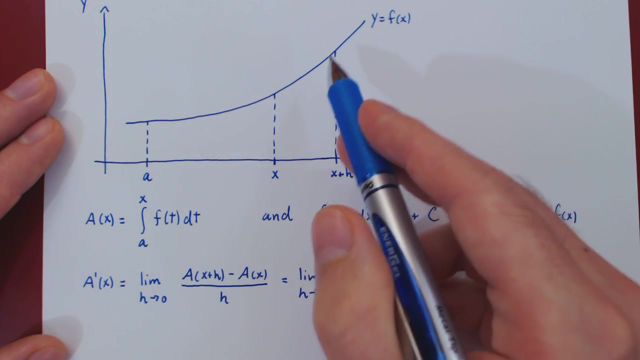 And for argument's sake let's assume that h is a positive number now. So x plus h will be slightly bigger than x, And now we have a second region. So the area function at x plus h is the area under f between a and x plus h. 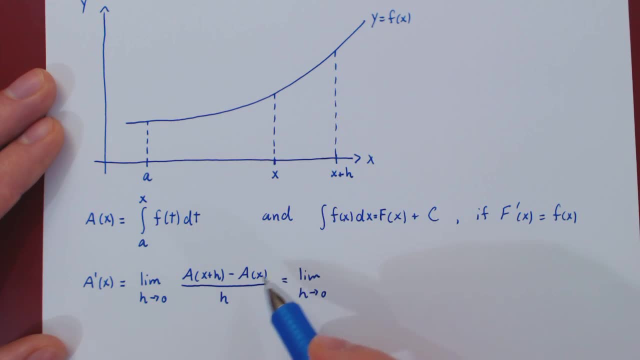 So it's the area of the larger region. But a of x is the area under f between a and x, So the area of the first and smaller region. So if you add the area of the larger region and then subtract the area of the first and smaller region, 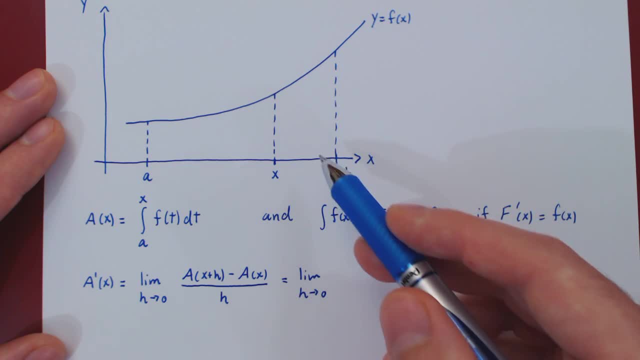 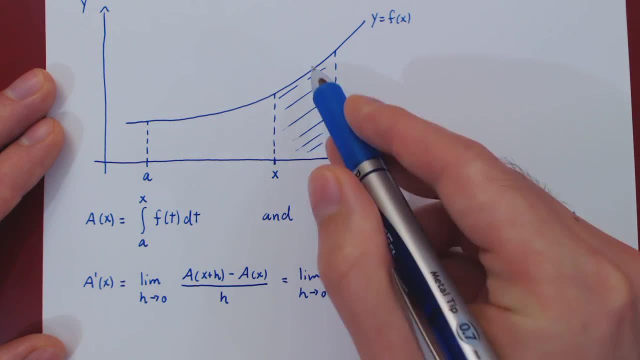 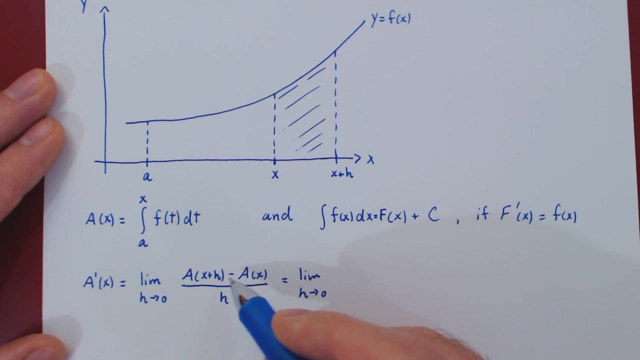 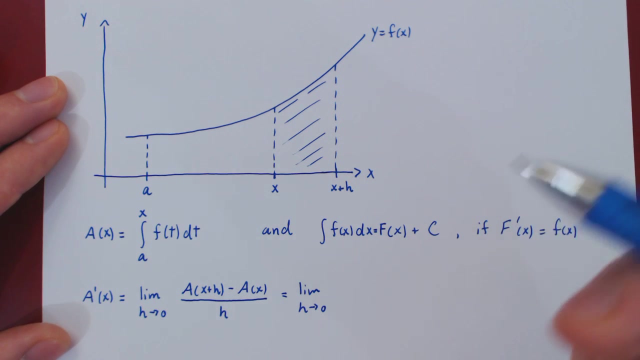 you're, of course, left with the area of the second. So the area of this now is exactly the numerator of our fraction, And our goal will be to find a simpler way of obtaining this area. And if you think of simple area, well, you have to think, of course, of the simplest possible shape. 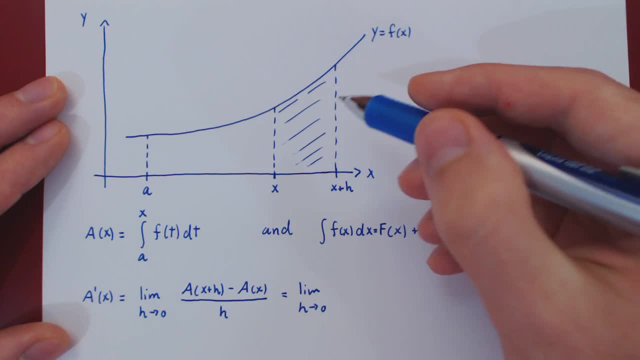 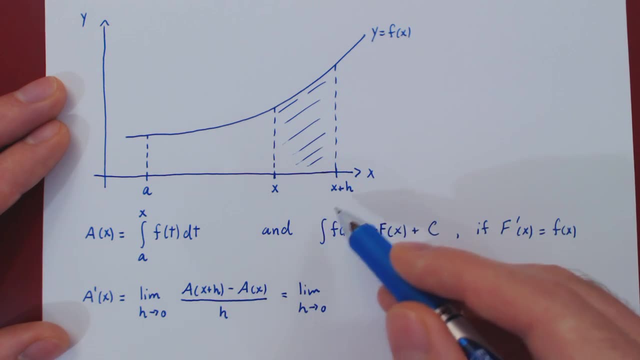 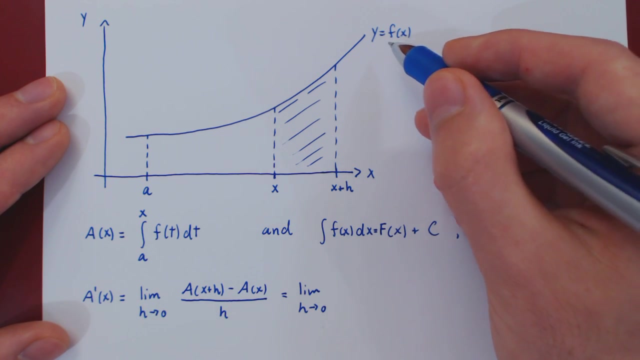 and that is of course a rectangle. So the question is here: can we find a rectangle whose area will be exactly equal to the area below f, between x and x plus h? So let's try and figure this out. And the idea depends here on the fact that f is continuous. 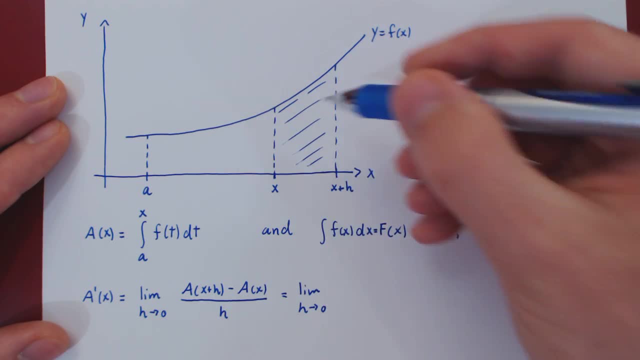 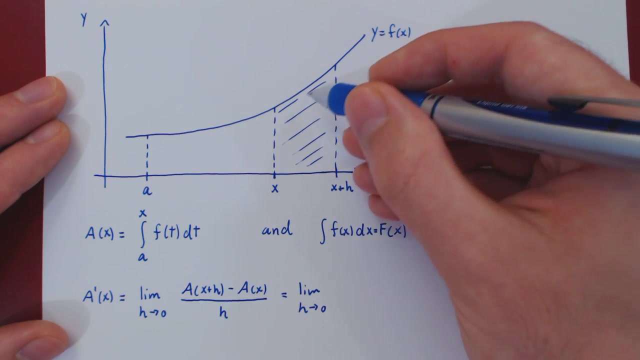 so that there is no break in the function. So suppose we pick this point to give us the height of our rectangle. So imagine we draw the corresponding rectangle and the rectangle now will be clearly too short. Its area will clearly be smaller than the exact area under f. 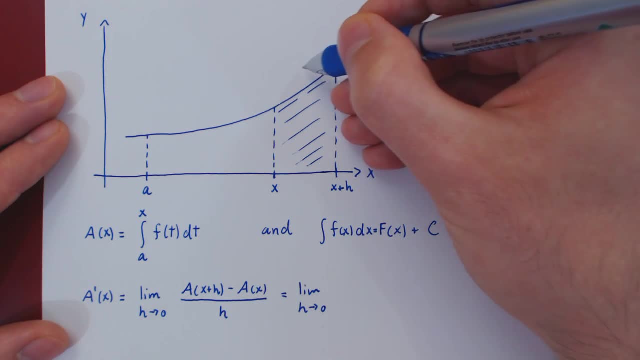 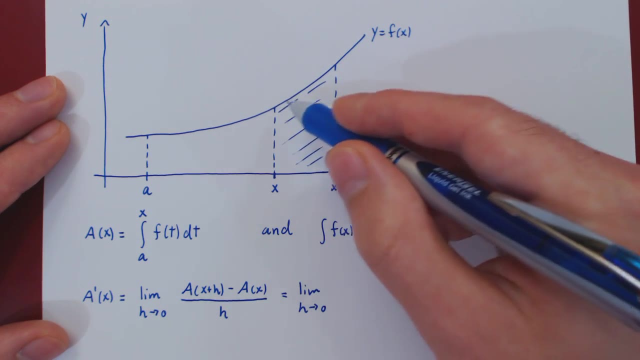 If we draw the corresponding rectangle. if we take this point to yield the height of our rectangle, then the rectangle will be too large and its area will clearly be larger than the area under f. But there has to be a sweet point between one that is too small. 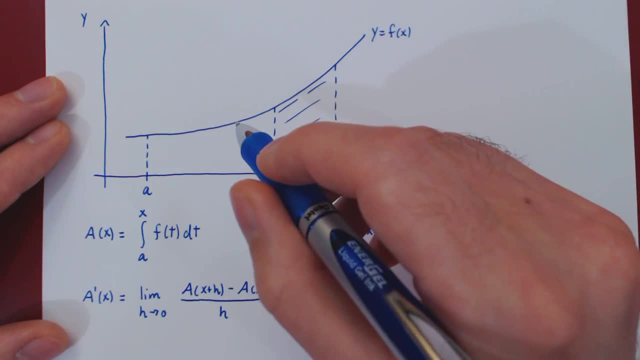 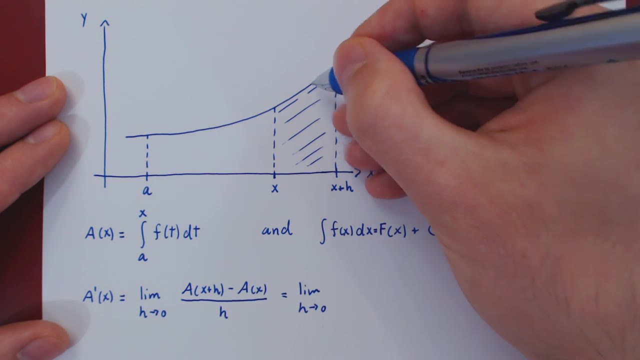 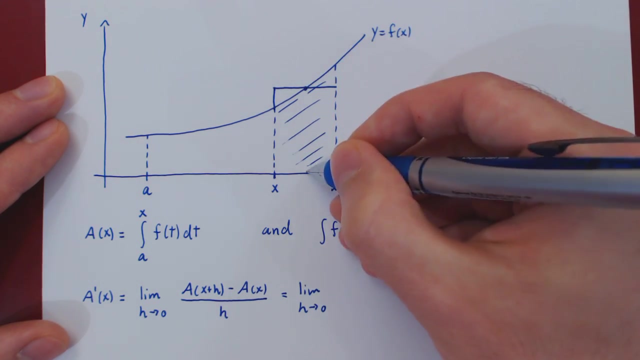 and one that is too large, where the height is just right, so that the area of the rectangle is exactly the area under f. You can try and visualize it. It looks like it would be this point and call this point x-hat. 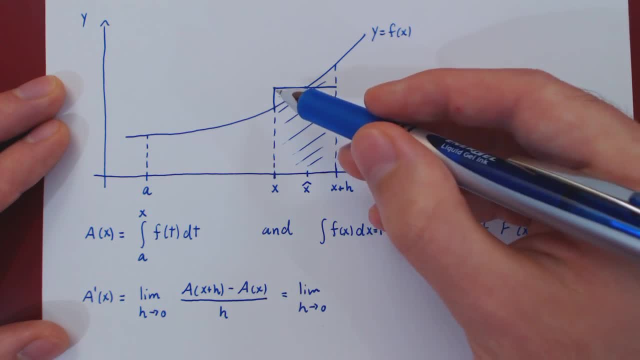 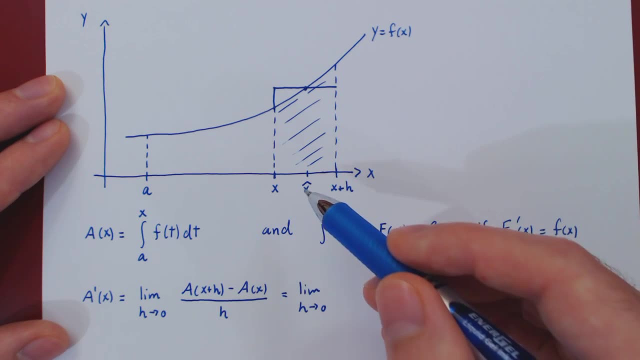 And you can kind of see it right, Thinking of the area of the rectangle, so the area of this piece, So let's break it down into two parts: The area from x to x-hat, then x-hat to x plus h. 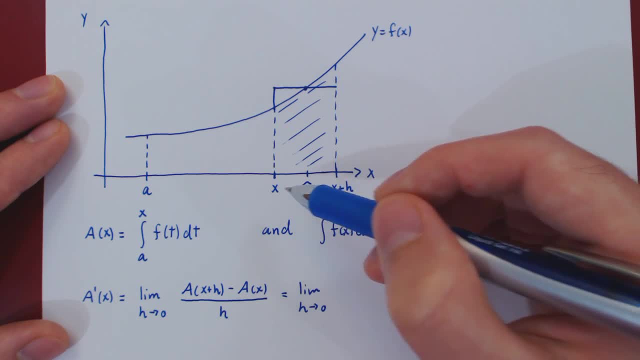 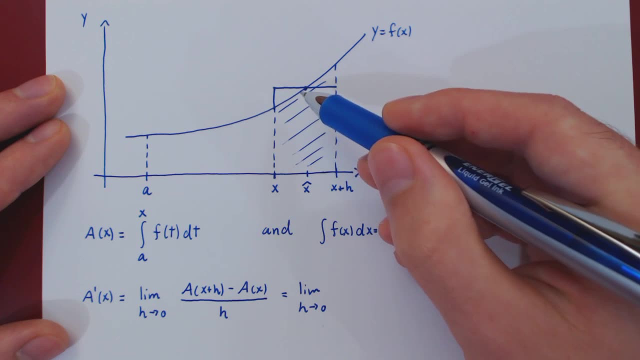 So if you compare the area from between x and x from the rectangle, then you have clearly more area in the rectangle than you have under the curve. But as you go from x-hat to x plus h, then the area under the rectangle is clearly smaller than the area under f. 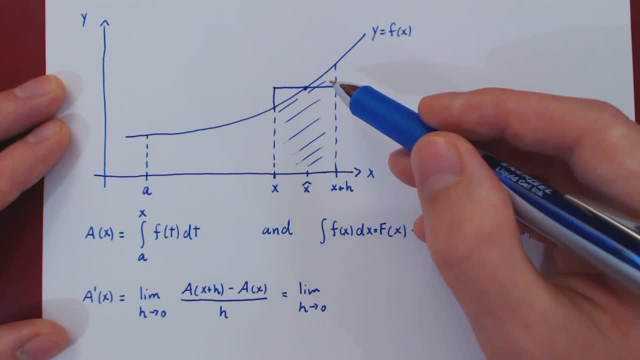 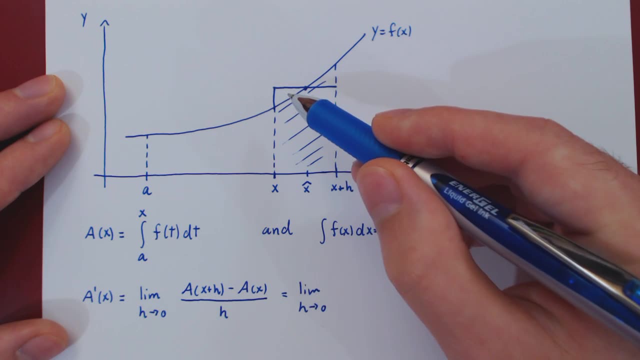 So what you're getting extra in the rectangle here, you're missing here And you can kind of see it if you choose the point x-hat, just right, What you have too much in terms of area from the rectangle is exactly the same as what you're missing. 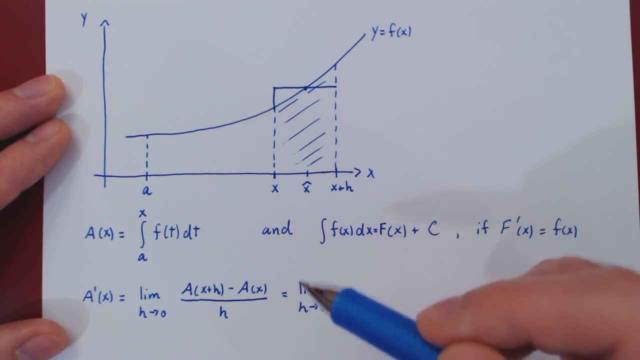 in terms of area from the rectangle. And so, with the right choice, the area of the rectangle will be exactly the same as the area below f. So now we ask: well, what is the area of the rectangle? Well, the area of the rectangle is nothing but the base times the height. 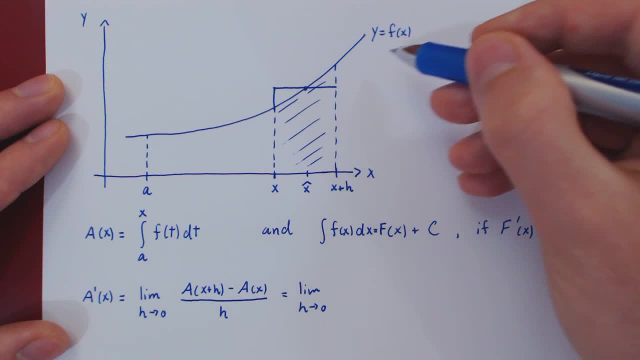 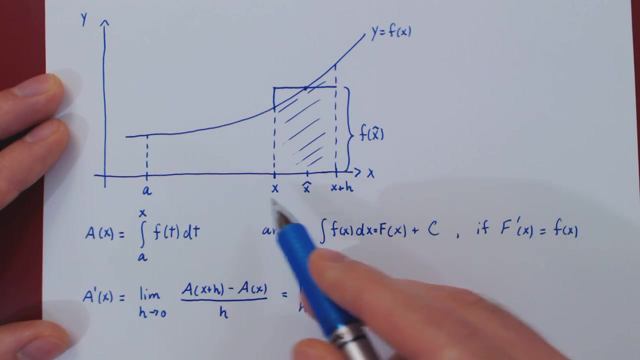 So what is the height? Well, the y-value on the curve f of, therefore, f of x-hat, is the height of our rectangle And the width of the rectangle, well, change in x. so x plus h minus x. 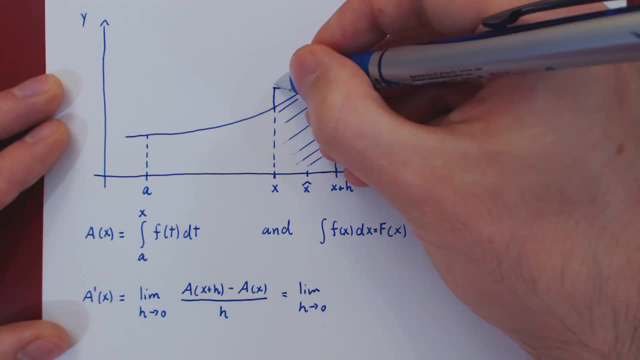 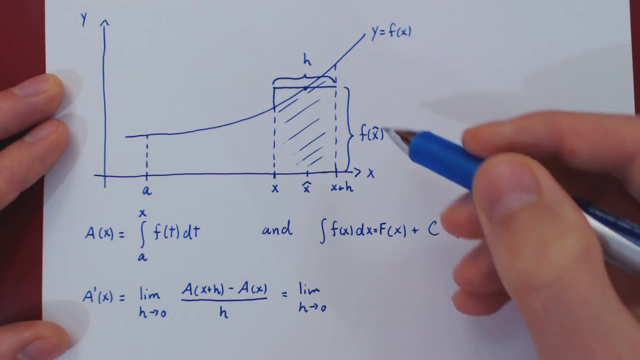 is, of course, simply h. So we have a rectangle whose area is f of x-hat times h. And now things are getting interesting. We can cancel the h over h And we're left with, quite simply, the limit, as h goes to 0. 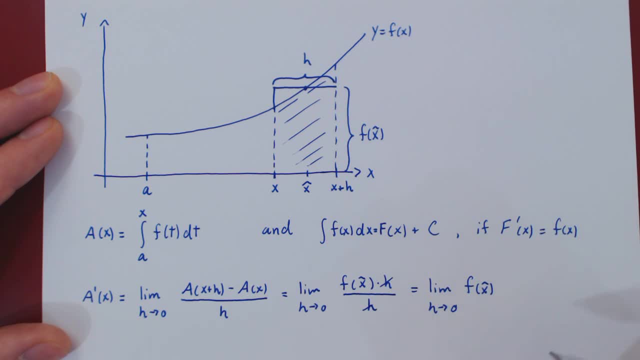 of f of x-hat And this limit. if you go back to the position of x-hat between x and x plus h, it will become apparent that this limit is now trivial. Right, we are letting h approach 0.. As h approaches 0,. 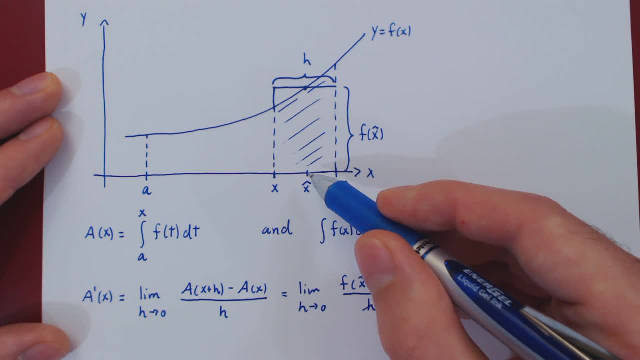 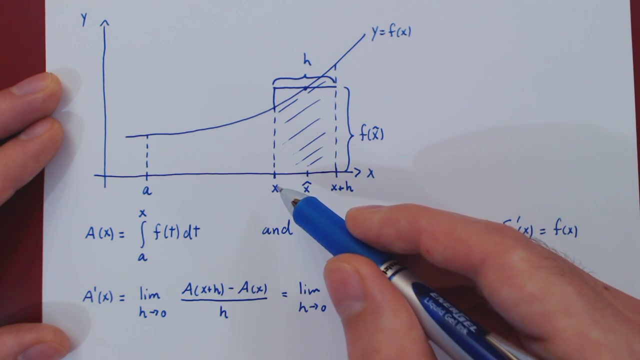 then x plus h will be approaching x. But as x-hat is always between x and x plus h, then as h goes to 0, this point will go to x, so it will push x-hat also onto x. So by the squeeze theorem, 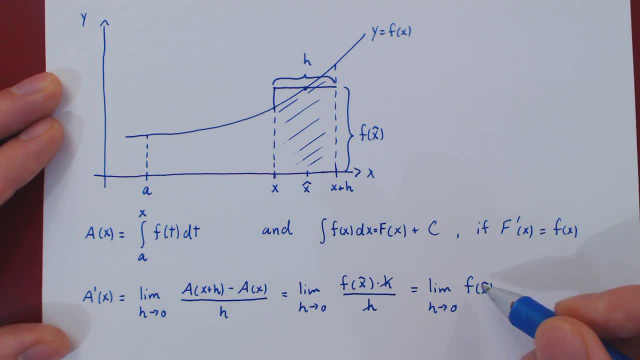 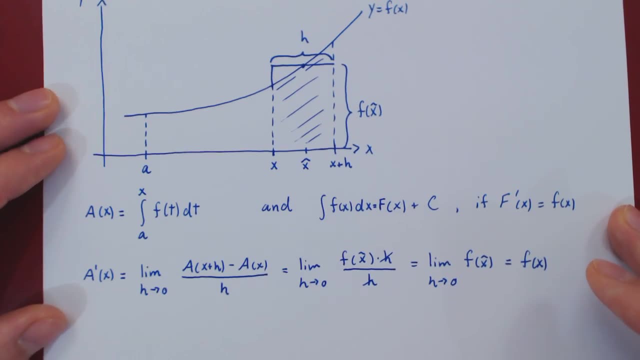 x-hat must converge to x and by continuity, f of x-hat will have to converge to in the limit f of x. And now things are getting really interesting, because what have we proved? The derivative of the area function. 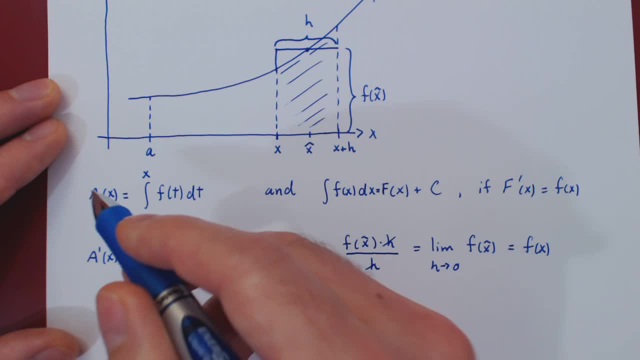 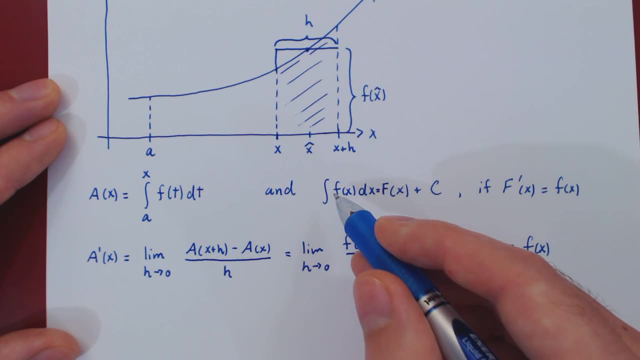 is lowercase f, So a of x is an antiderivative to lowercase f of x. But all antiderivatives to lowercase f must be of the form uppercase f plus a constant, As a of x is an antiderivative to lowercase f of x. 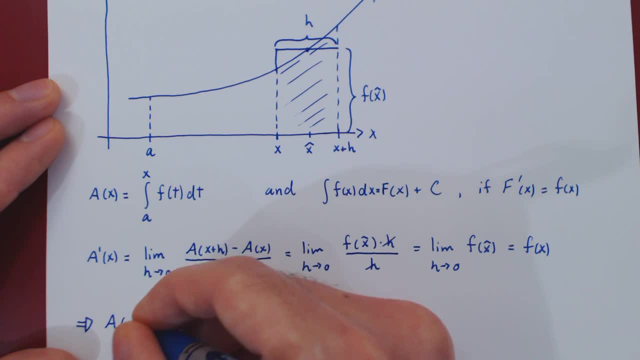 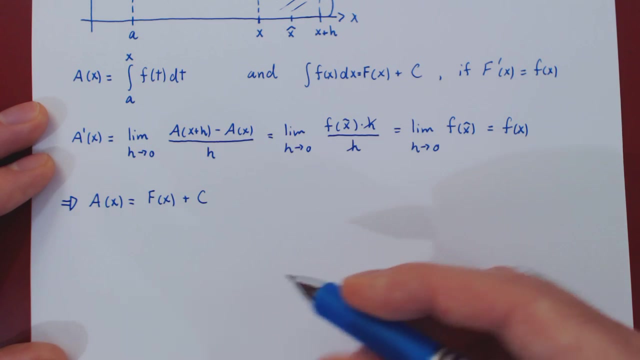 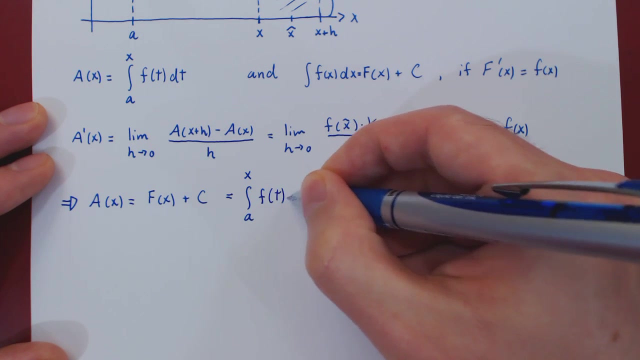 uppercase a of x. the area function has to be uppercase f of x plus some constant. And now let's write back the area function in terms of the definite integral And you'll see that we're just about done now. So we have the integral of f from a to x. 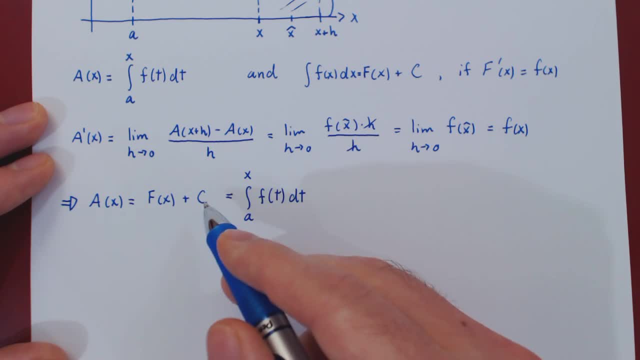 is f of x plus c. Well, c is this unknown constant. to solve for an unknown constant you need an equation. The equality here is true for any choice of x. so can we choose a value of x that will make the equality become trivial. 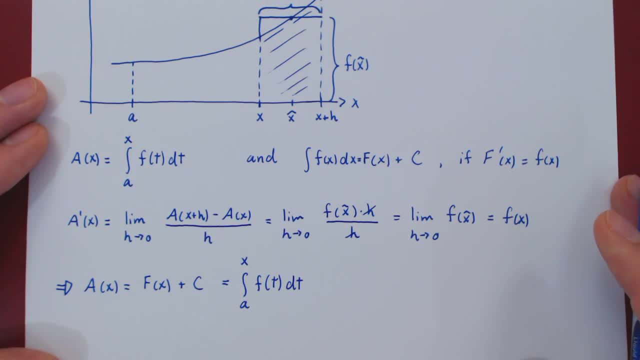 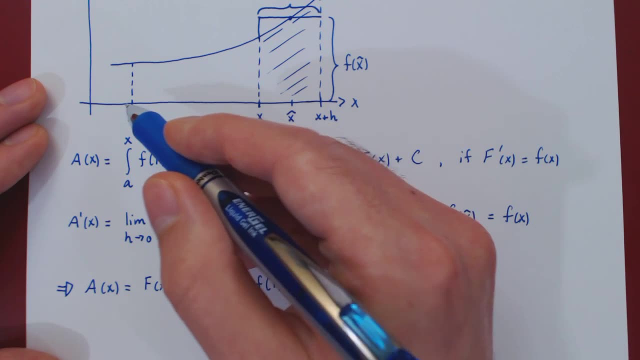 so we can solve for c? And the answer is yes. How can we make this trivial? Well, if you choose x to be equal to a, then the interval from a to a consists of a single point. therefore, we have no region. 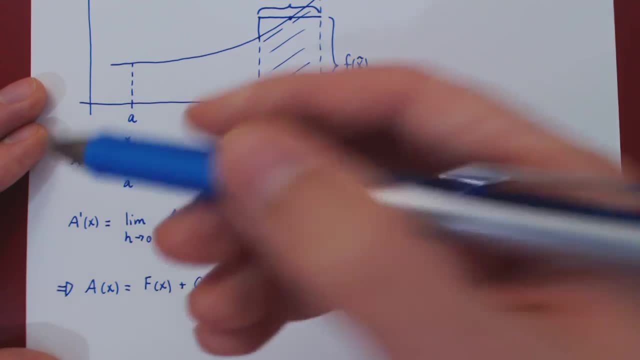 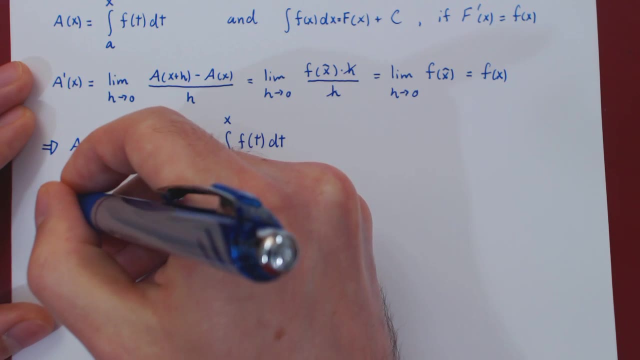 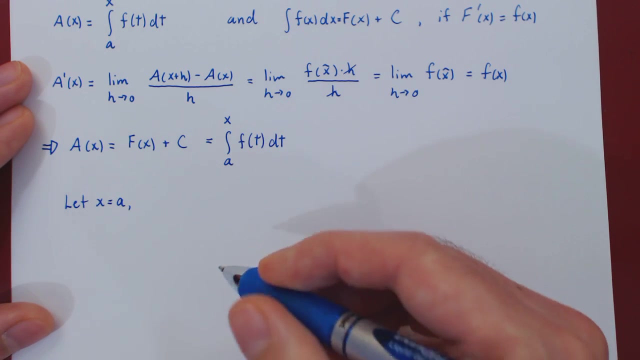 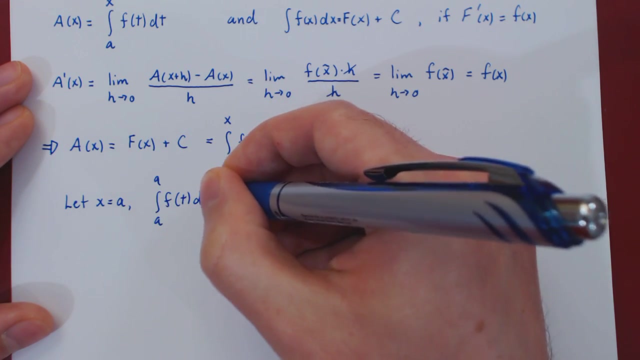 just a vertical line segment and the area of a line of course is zero. So here the key in solving for c is letting x to be equal to a. Then let me write this first: so the integral from a to a of f of t, dt. 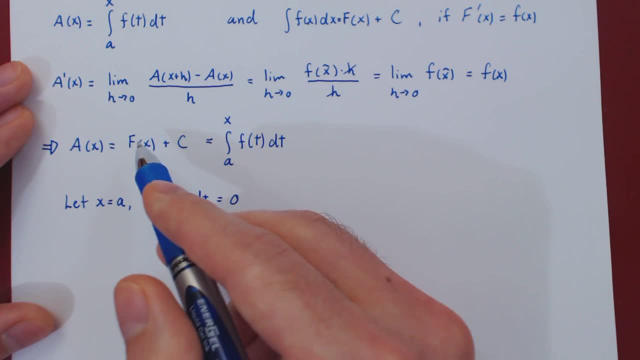 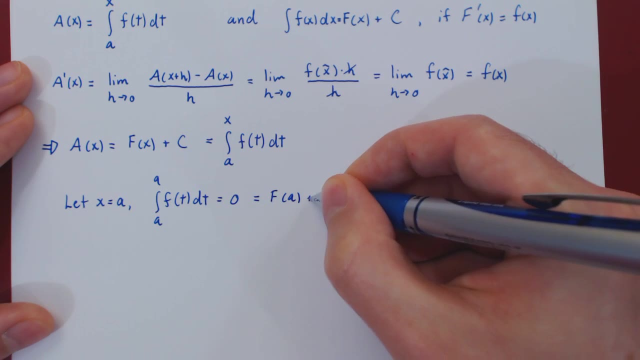 is equal to zero. there is no area now, and this, when x is a, is f of a plus c. So you can isolate c by subtracting f of a. therefore c is nothing but the negative of f of a. So now we can replace c. 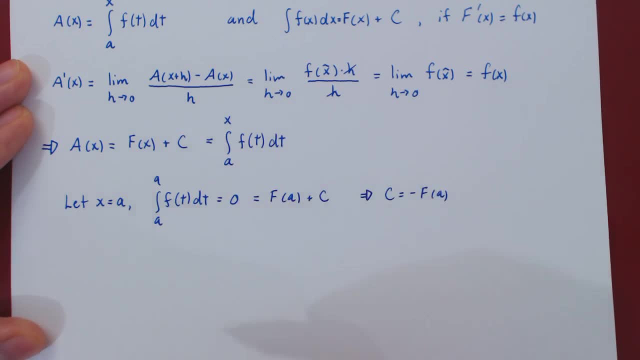 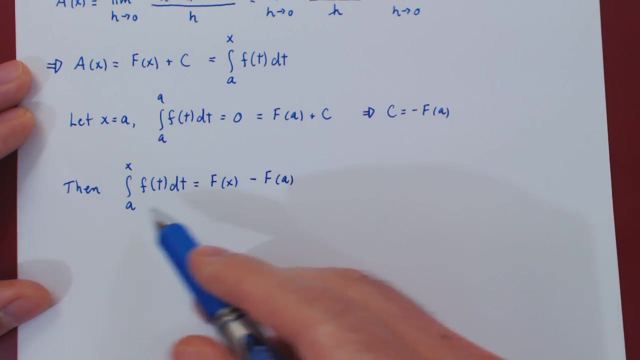 in the original equality. Let me write first a definite integral. So this equals f of x plus c, but again c is negative f of a. And now think about this: This is valid for any choice of x, So we can replace x by any constant of our choice. 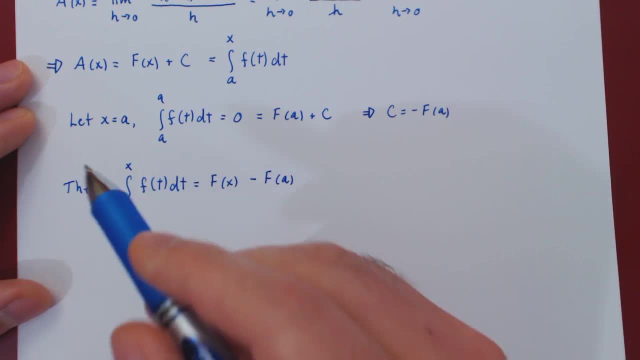 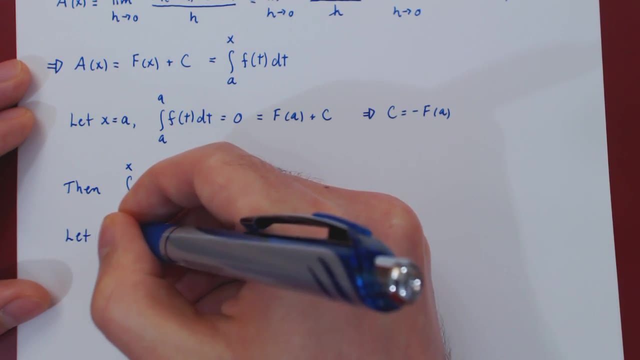 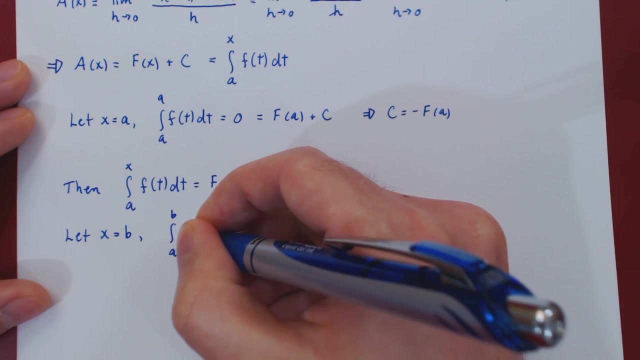 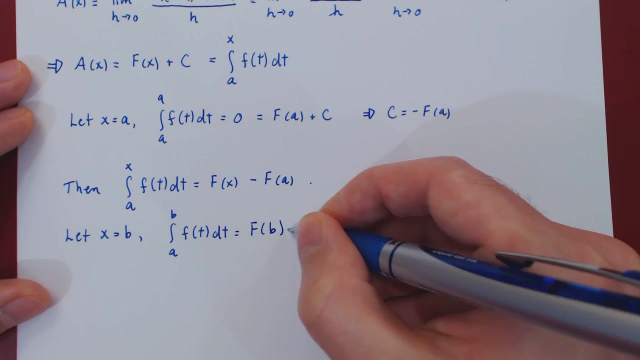 and the equality is still valid. So let's replace x by the familiar constant b. So what will this become? Well, the integral from a to b, of f, of t, dt, equals f of b minus f of a, And we now have the familiar form. 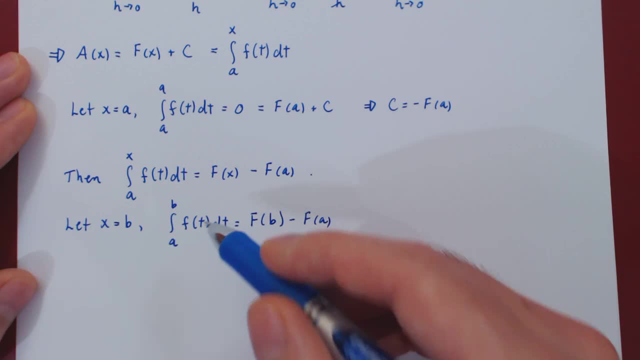 of the fundamental theorem of calculus. The only difference is that we are now using t instead of the more familiar x, but we can now go from t back to x. if you look, there are no longer any x's in the expression. So we can now replace t by any variable of our choice. 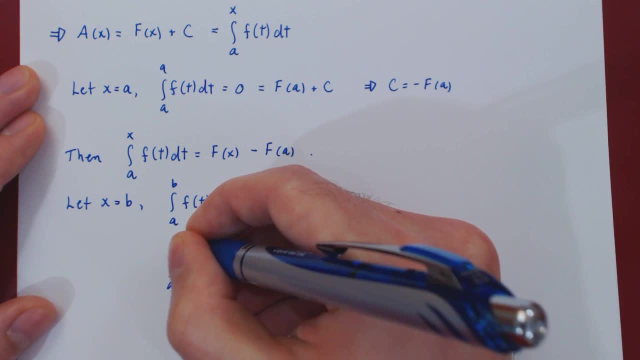 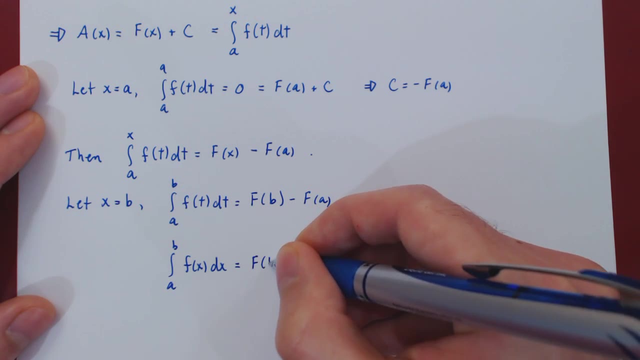 and so we go with again the familiar choice of x. So the integral from a to b, of f, of x, dx is its antiderivative at b minus its antiderivative at a, And we now have the familiar form of the fundamental theorem of calculus. 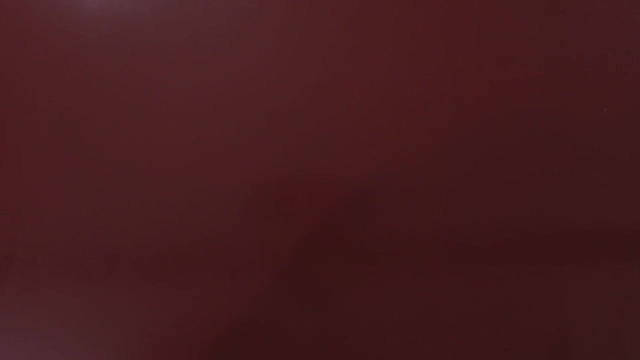 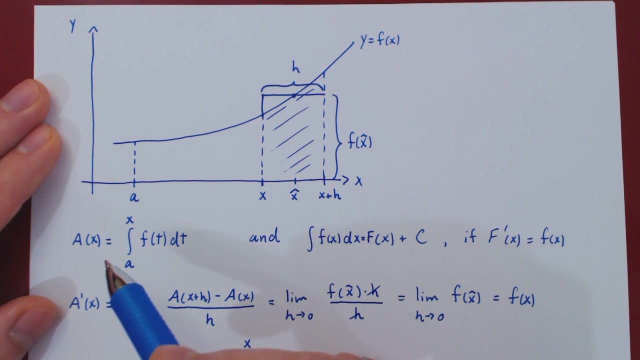 And if we summarize the proof, it boils down to two essential facts. The first is that antiderivatives are unique up to the addition of a constant. We then constructed an area function and then showed, using a beautiful geometric argument, that the area function was an antiderivative. 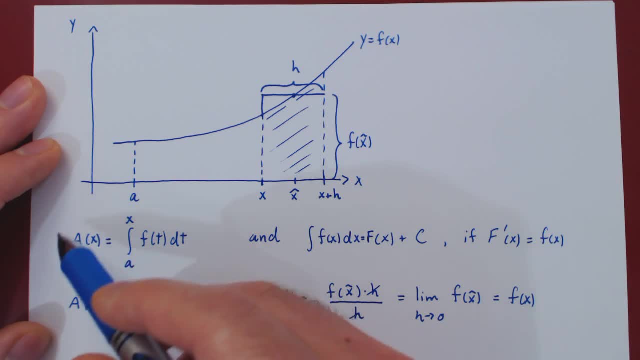 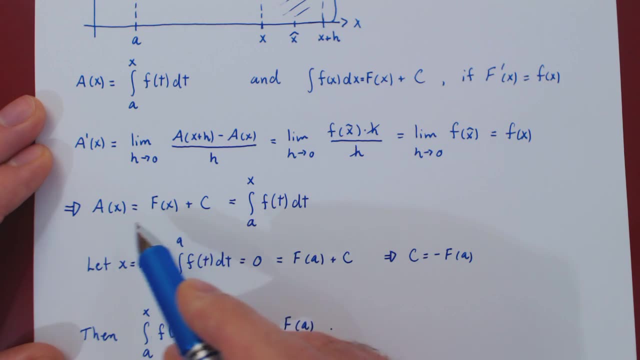 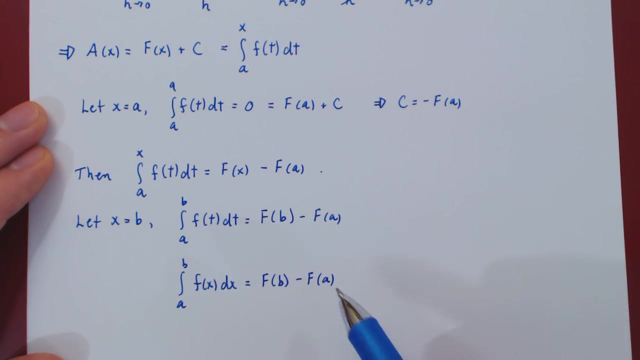 to the original function. so a of x being an antiderivative to lowercase f had to be of the form f of x plus c, And then it was routine to solve for c, and from this we obtained directly the fundamental theorem of calculus. 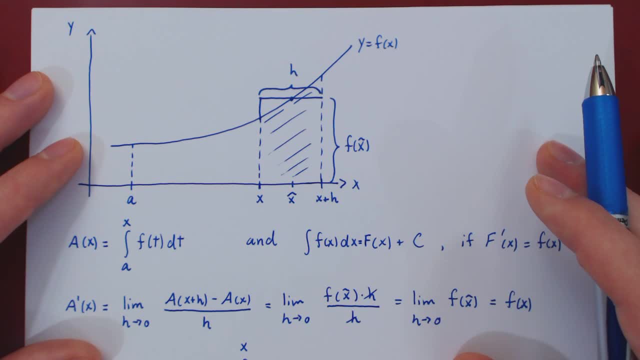 So hopefully you appreciate this rather simple and elegant proof. 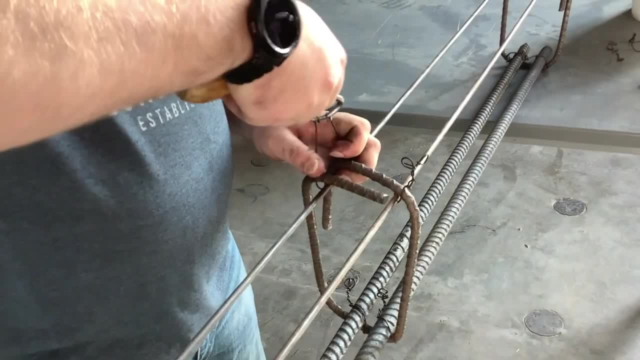 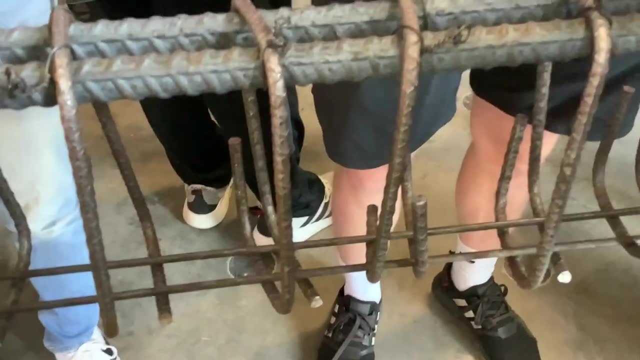 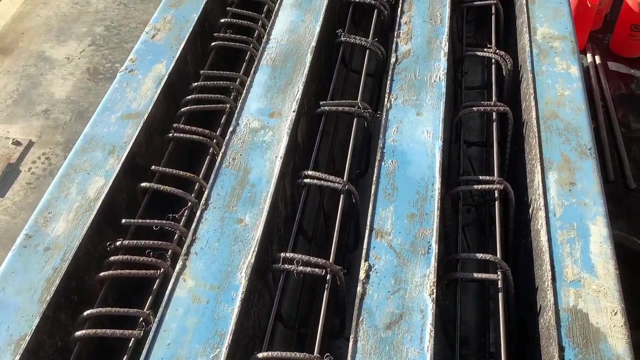 we made reinforced concrete beams in our lab to see how much load will these things carry and how will they break. so we went through the whole fabrication process: tying our rebar cages, boiling up the forms, dropping the cages into the forms, and now we have six beams ready to cast. 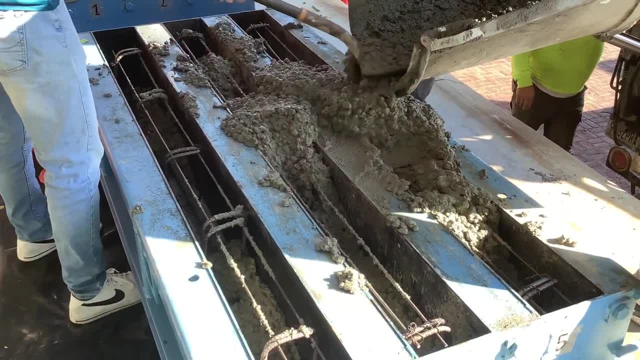 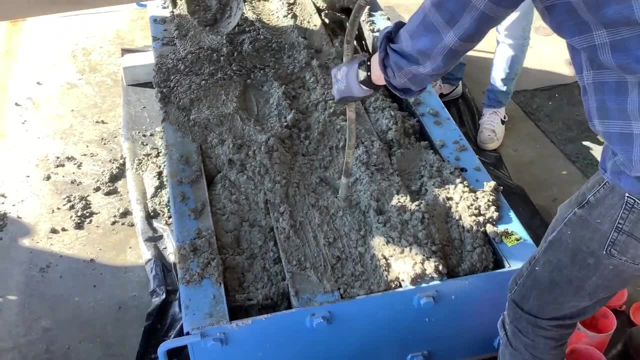 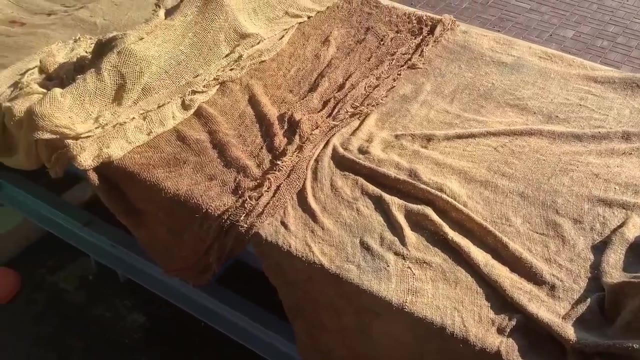 so, of course, what is reinforced concrete without the concrete? we've got to fill our forms and also check the slump to make sure that everything is looking good, casting some cylinders to check the strength and vibrating everything into place, putting on the finishing touches and then curing for seven days when we pull it out of the forms. here is the final product, ready to test. 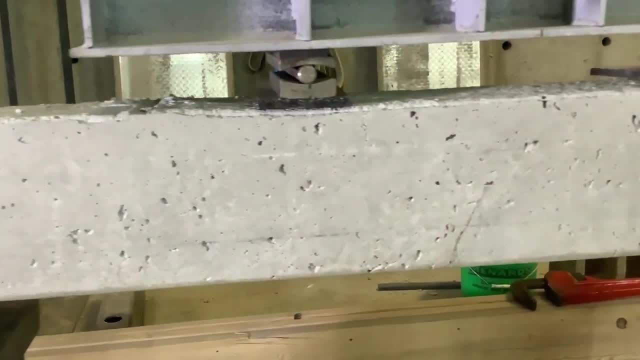 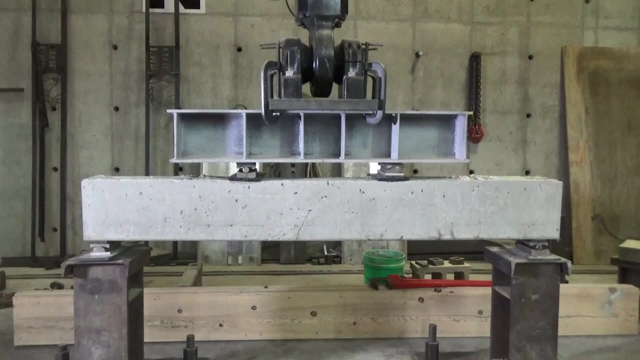 under our actuator. let's look at the results of these tests and see how they work. before we break that first beam, let's check out our testing setup. so our main load is going to be applied by our actuator- let's call that load p- and it's going to be divided in half by our spreader beam.